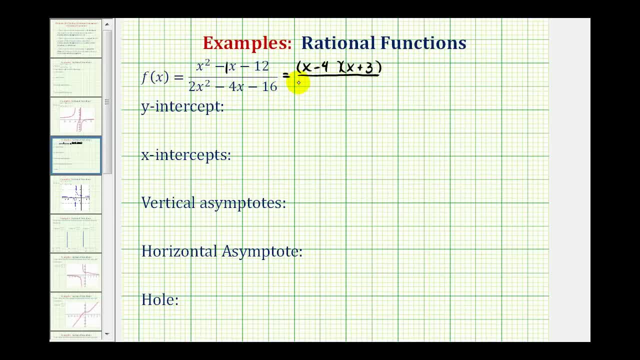 Looking at the denominator, notice how we first have a common factor of two. Let's factor two out. That would give us x squared minus two, x minus eight, but this does factor again. We still have our factor of two, and then we'll have two binomial factors. 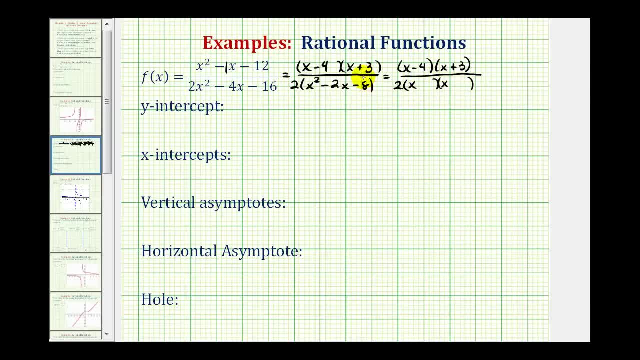 The factors of x squared are x and x. The factors of negative eight that add to negative two are negative four and positive two. One of the reasons it's important to factor our rational functions is notice. in this case we have a common factor of x minus four between the numerator and denominator. 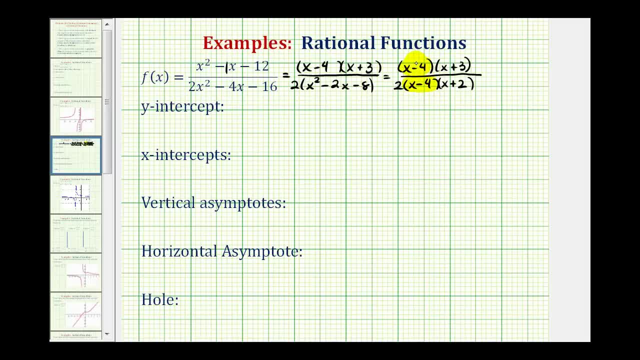 The reason this is important is that the values of x that make this common factor equal to zero will not give us an x-intercept or a vertical asymptote. It's actually going to give us a hole Again, since four makes this factor equal to zero. 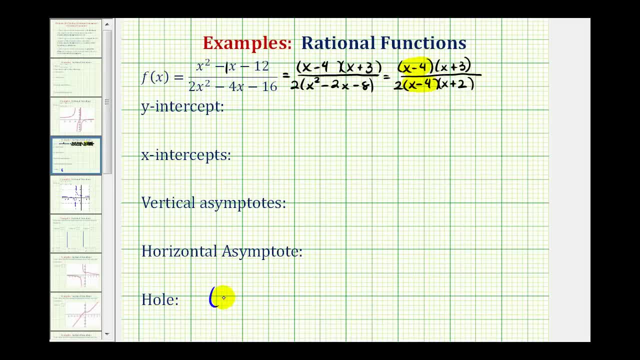 that means we're going to have a hole at the point where the x-coordinate is equal to four. Once we know that, we can start to calculate our rational functions. Once we know this, we can go ahead and simplify the function, meaning simplify out this common factor. 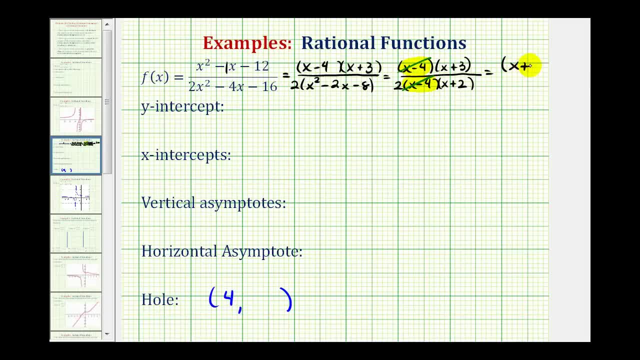 leaving us with the function: the quantity x plus three divided by two times the quantity x plus two. The graph of this simplified function will be exactly the same as the graph of the original function, except there will be a hole at x equals four. 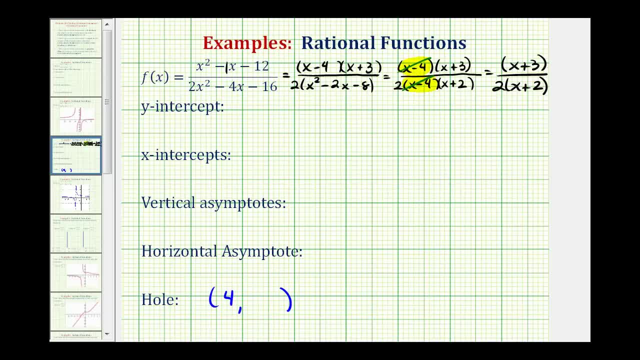 Now to determine the y-coordinate of where this hole will be. we can now evaluate the simplified function at: x equals four, So f of four of the simplified function would be four plus three. divided by, we'd have two times four plus two. This is going to be seven. this will be six times two or 12.. 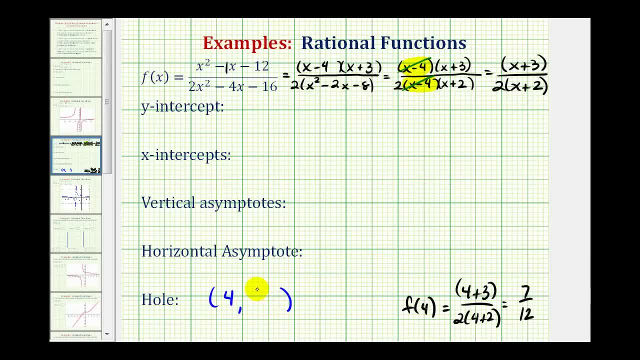 So there'll be a hole in the graph at the point four comma seven twelfths. Now that we have a hole here, we can use the simplified function here to determine the rest of the information, So to find the y-intercept of our function. 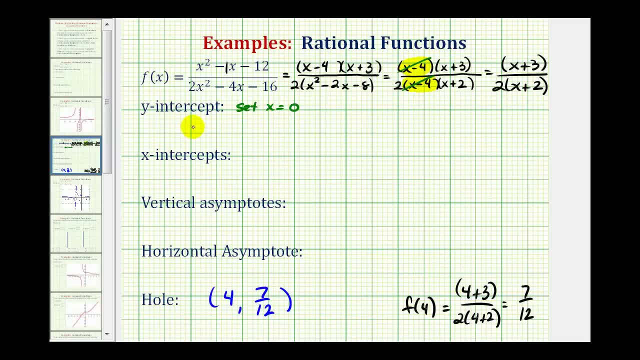 we'll set x equal to zero, which means we need to evaluate f of zero and we can go ahead and use the simplified function. So if x is zero, we would have three all over two times two, which is four. So f of zero equals three fourths. 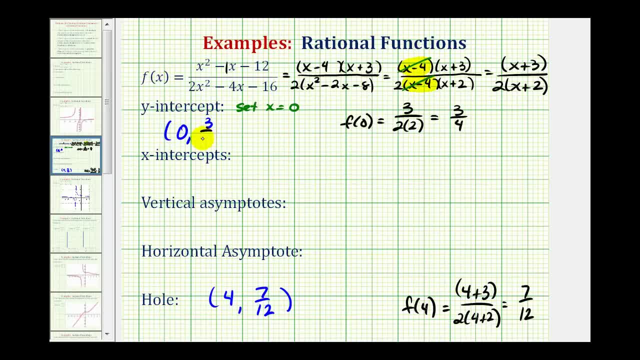 which means the y-intercept is the point zero. three fourths Now. to determine the x-intercepts, we set y or f of x equal to zero, And again we're going to use the simplified function And because we have a rational function, 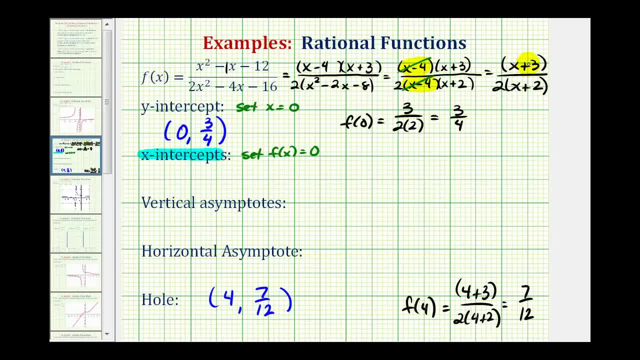 this function is only going to equal zero when the numerator is equal to zero. Notice, the numerator will equal zero when x equals negative three, which means our x-intercept is the point, negative three, zero. Notice, if we did not use the simplified function. 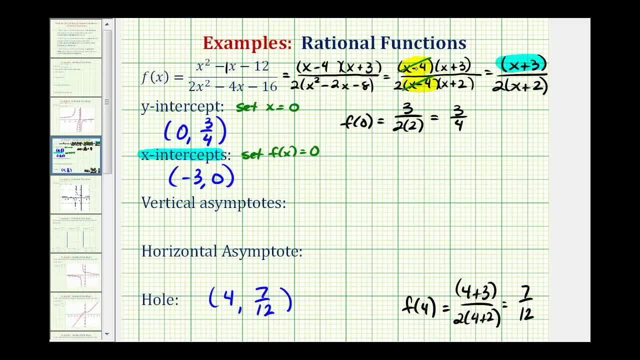 we would make the mistake and assume there would be an x-intercept when x equals four. but there's not going to be because the function is undefined at four and there's actually a hole in the function. That's why we have to use the simplified function. 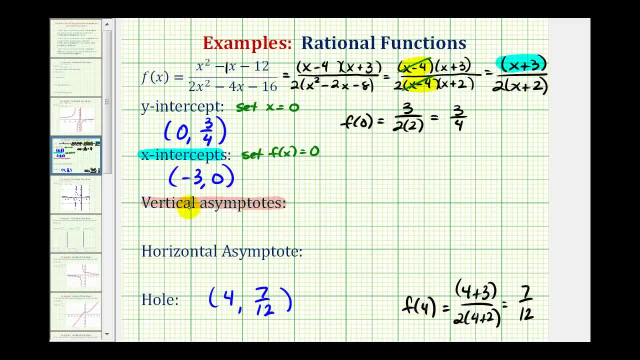 And then to determine the vertical asymptotes. these occur when the denominator is equal to zero. So x plus two is equal to zero when x equals negative two. Therefore, the equation of the vertical asymptote is: x equals negative two. And now for the last question. 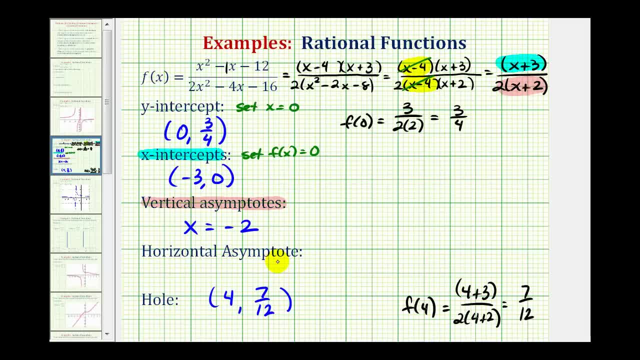 we want to determine the horizontal asymptotes which can be found by analyzing the degree of the numerator and denominator, And we can use the simplified function or the original function Notice in this form: here the numerator and denominator have degree one and since they have the same degree, 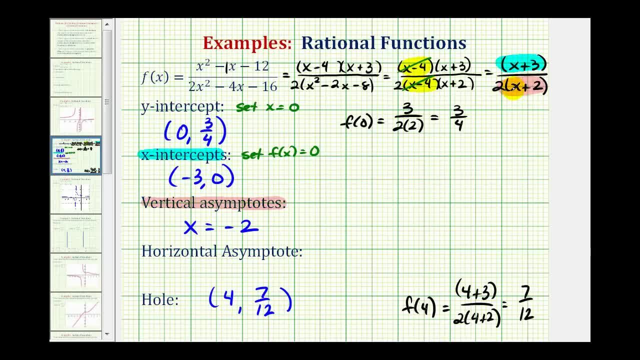 the equation of the horizontal asymptote will be: y equals the ratio of the leading coefficients. Notice: the leading coefficient of the numerator would be one. leading coefficient of the denominator would be two. So y equals one over two or y equals one half. 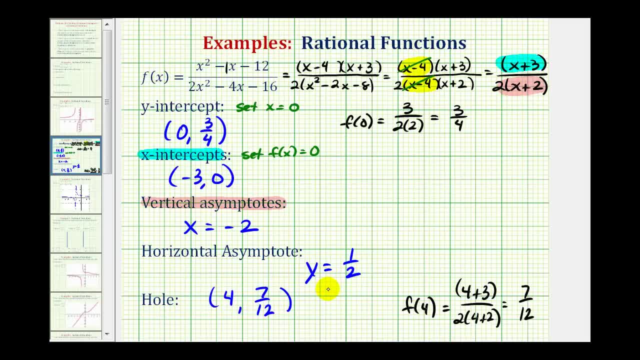 is the equation of the horizontal asymptote. Using this shortcut, remember: if the degree of the numerator was less than the degree of the denominator, then the horizontal asymptote would be: y equals zero, And if the degree of the numerator was greater than the degree of the denominator, 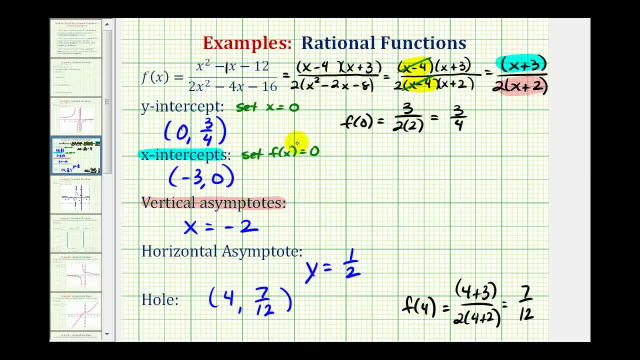 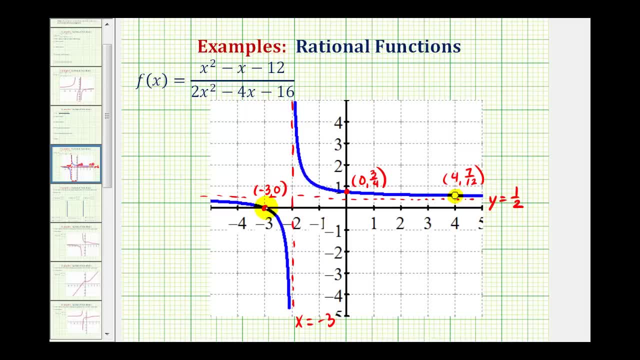 there would be no horizontal asymptote. Let's go ahead and verify our work by graphing the function. Here's the hole in the function at x equals four. Here's our x intercept of negative three. our y intercept of three fourths.